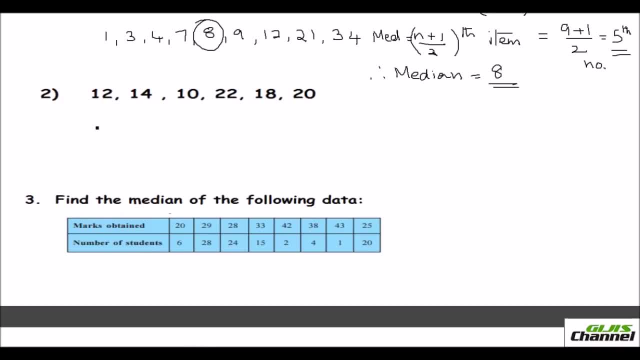 numbers here, but here I have only 6 numbers, So 6 is an even number. I told you you have to arrange it first. Okay, Now that we have arranged it, find out what is your n? n is 6.. So that is. 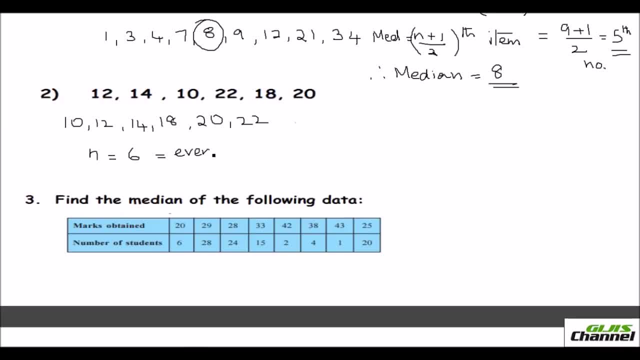 even Okay, When it is even what you need to do is you have to find out the average of you. find out what is n by 2.. Okay, So that is 6 by 2 is third number. So that's third number Also find. 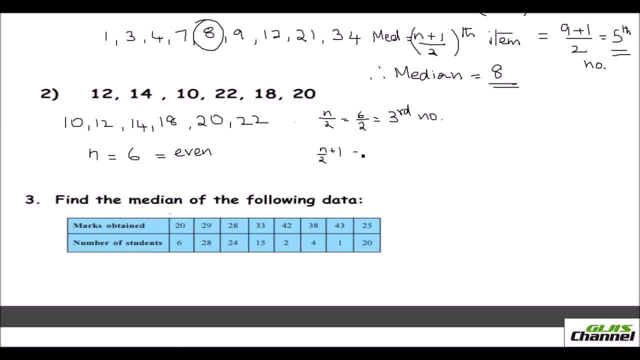 out n by 2 plus 1 number. Okay, So that will be fourth number. Okay, So n plus 1, it is not n over 2 plus 1.. Okay, It is not n plus 1 by 2.. You have to take the next number, that is, you got whatever. 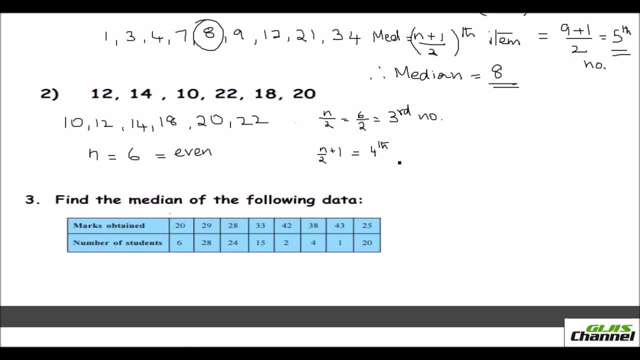 you got by doing n by 2.. The next number, Okay, Fourth number, and it's average. The average of these two number will be your median. So median is equal to. third number is what? 14.. Right, This is equal to 14 and the 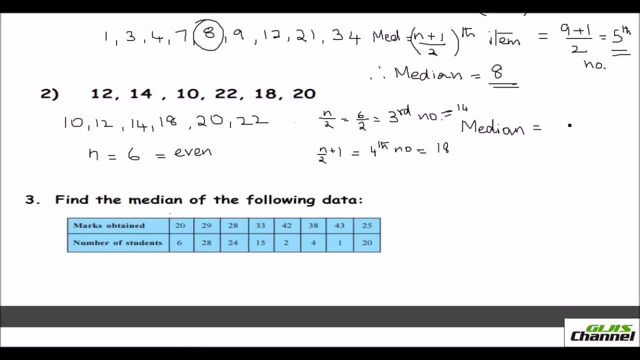 fourth number here is 18.. So median will be 14 plus 18 over 2.. Okay, So that will give you 32 over 2 and the median is 16.. 16 is your answer. Got it? So this is how. when the list of numbers 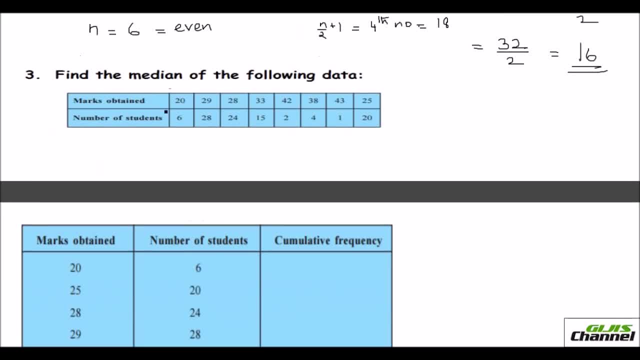 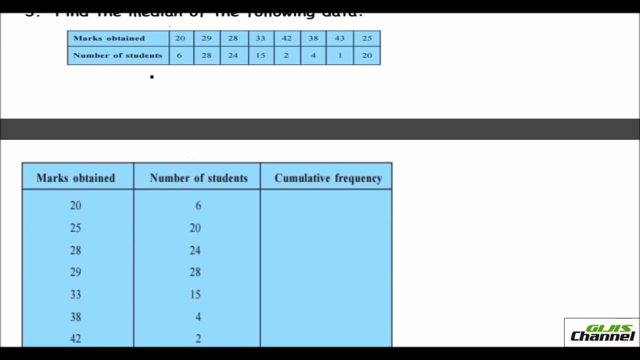 are given. But another type is that they would give you the marks obtained. Here, the marks obtained is given and also the frequency is given. The values and the frequency are given. Okay, So I will show you how to write. First of all, as I told you earlier, the marks obtained has to be written in ascending order, Okay. 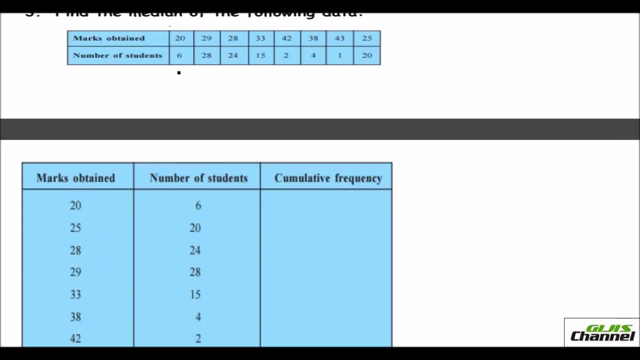 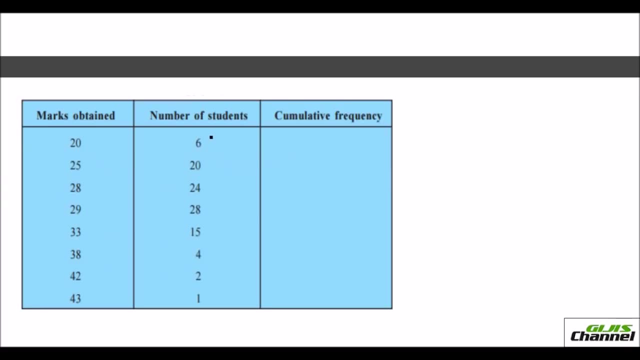 So I have written first 2,, 20 and the frequency: the corresponding frequency I have written here. Then it is after 20, it is 25 and the corresponding frequency here. Likewise. I have already arranged it. Now. what you need to do is: this is your x value, Okay, And this is your frequency value. 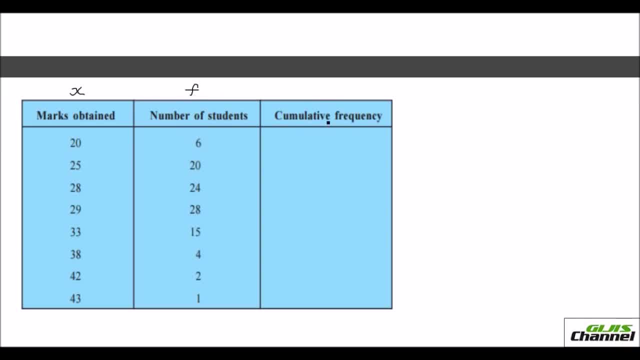 Understood. Now what you do is you find the cumulative frequency. Cumulative frequency is nothing but summing up the frequency at each step. Okay, Initially it is 6.. Then it is: you add 6 plus 20.. Okay, This 20.. So that will give you 26.. Then you will add 26 plus 24.. 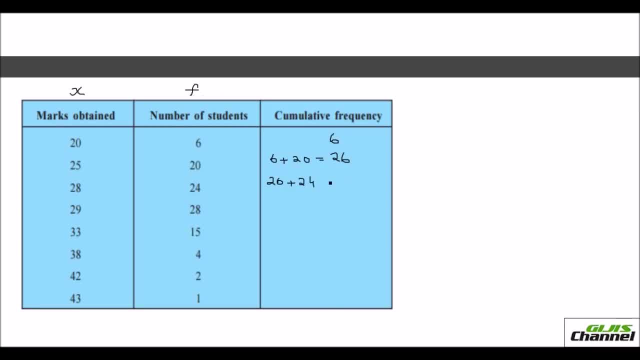 Okay, So that will give you 50. Next step is 50 plus 28.. Right, So that is 78. Then you have 78 plus 15, will give you 93.. Next is 93 plus 4.. 97.. 97 plus 2.. 99. And finally, 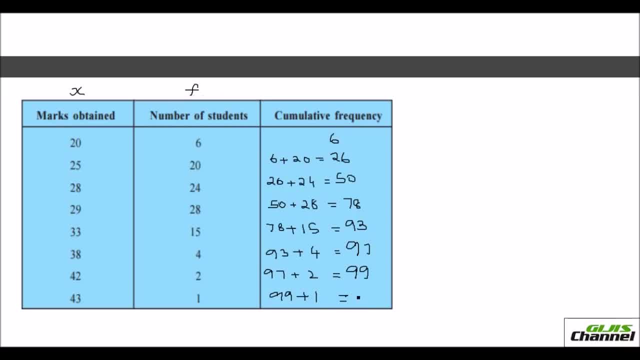 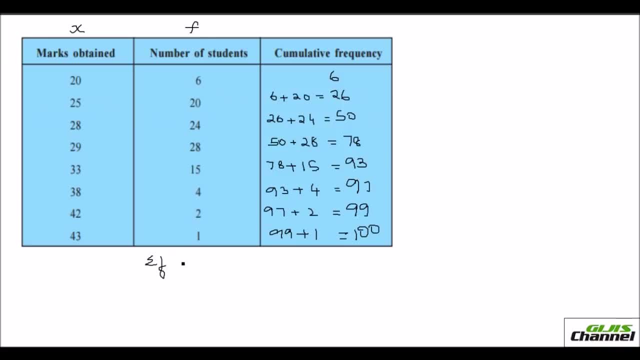 you have 99 plus 1. And that gives you 100.. Okay, Always see that this total of frequency will match with the last digit in the cumulative frequency. Okay, If you total this frequency, that will be equal to this last digit you get in the cumulative frequency, Did you get? 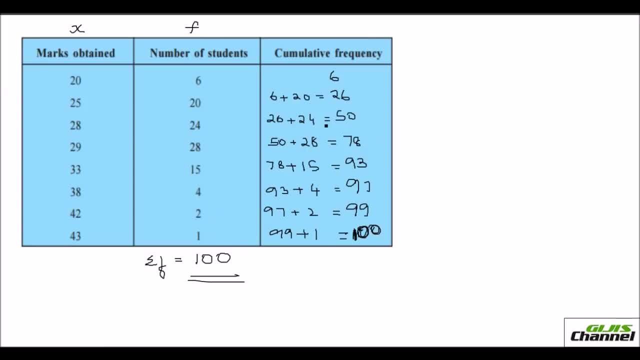 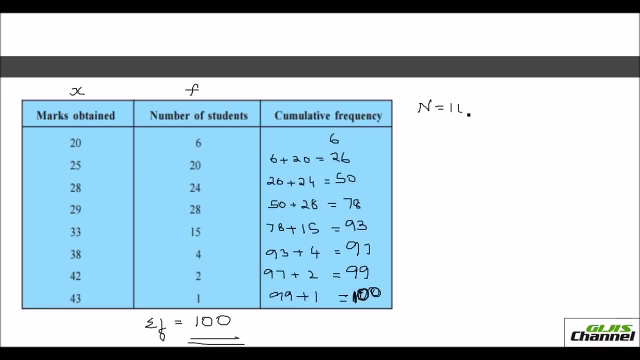 that Okay. Now your n. This time it is capital n, Because it is a total Right. So your n is 100.. So when n is 100, it means it is even Right. So when it is even, what do we do? We do n by 2.. 100 over 2 is 50th item And the next number you. 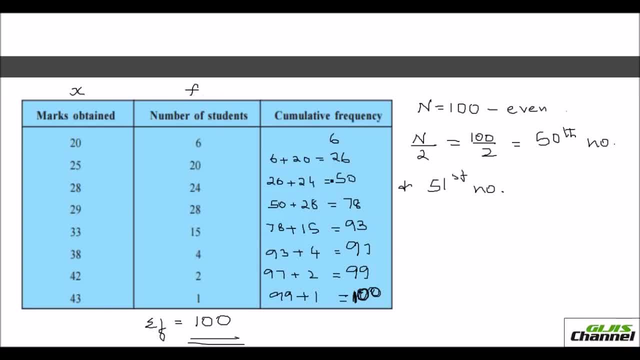 have to take Right 51st number. So here you see the 50. You just look at the cumulative frequency. Your 50th number Is Is 28.. Right, The x value is 28.. And the next number 51st number will be 29.. Right. 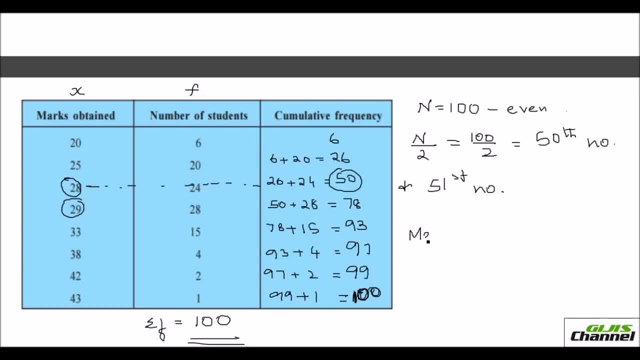 So you take, median will be the average of these two x values. Always median. you take from the x value. Okay, So the median will be 28 plus 29 over 2.. You are finding the average Right. So this will give you. 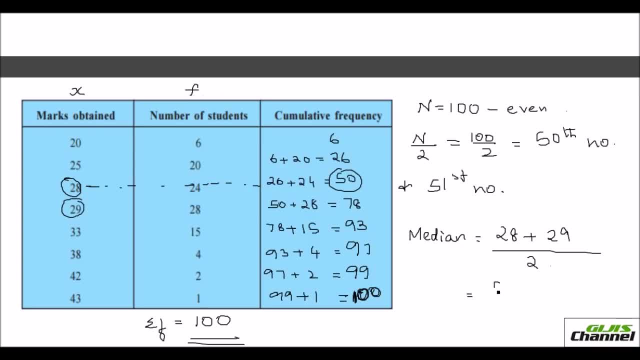 57.. Right, Yeah, 57 over 2.. And so your median is 28.5.. Isn't that easy. So this is when the x values and the frequency are given. Okay, Now I am going to do the grouped data. 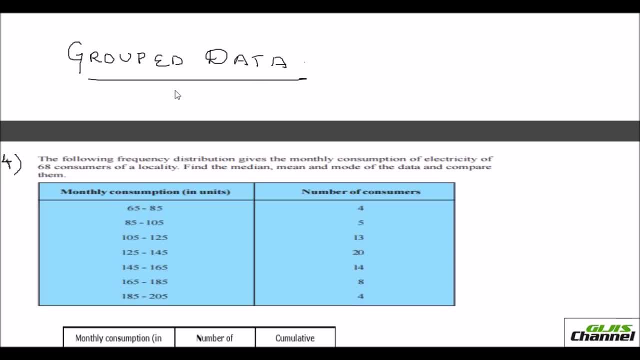 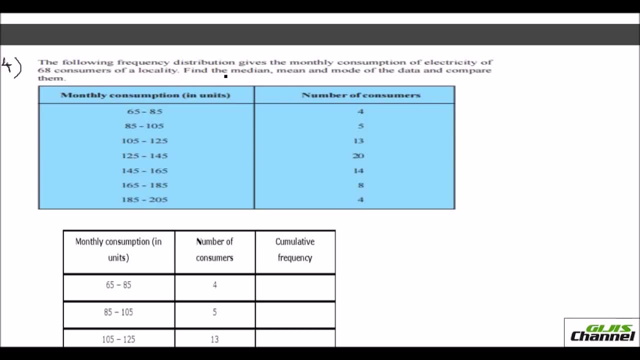 So long we were doing ungrouped data. Now this is grouped data which we are doing down Here. a question is given: given here the following frequency distribution gives the monthly consumption of electricity of 68 consumers of the locality. find the- let's just do the median alone here. find the median. 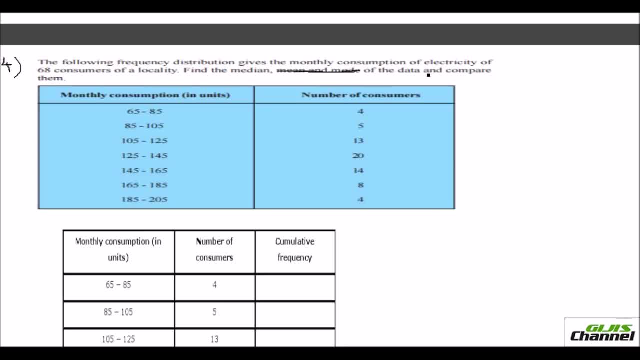 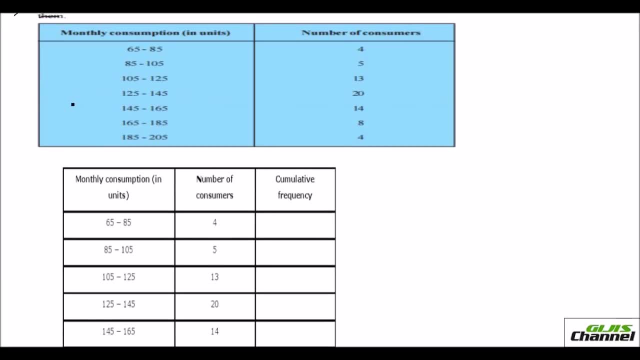 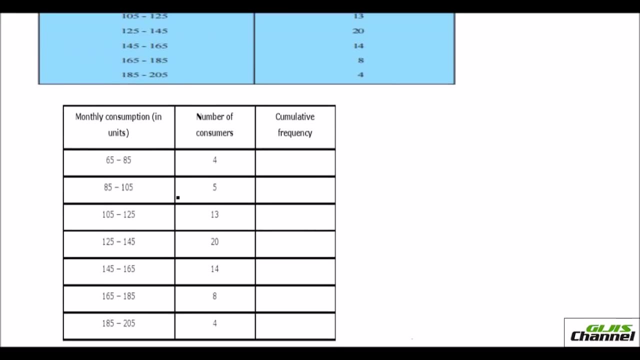 of the data. okay, okay, that will do. this is what we need to do now: just find the median. to find the median, i have rewritten this because, since you can see, the class interval is in the ascending order only, so i needn't change anything. i've just copied down. uh, those two columns. okay, 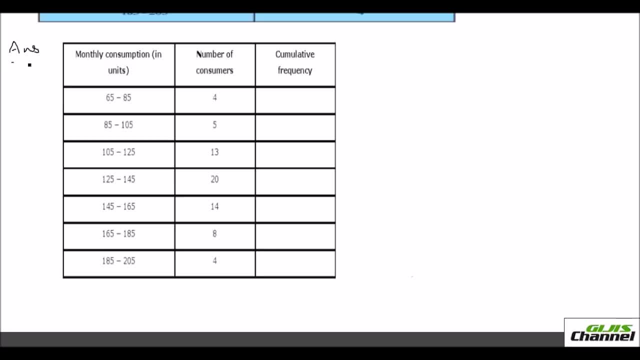 this is my answer and i have a third column to find the cumulative frequency. i hope you understood what is cumulative frequency. so first i would write 4, then it is 5 plus 4. next it is 9 plus 13. right, 9 plus 13 is 22, then you have to add 22. 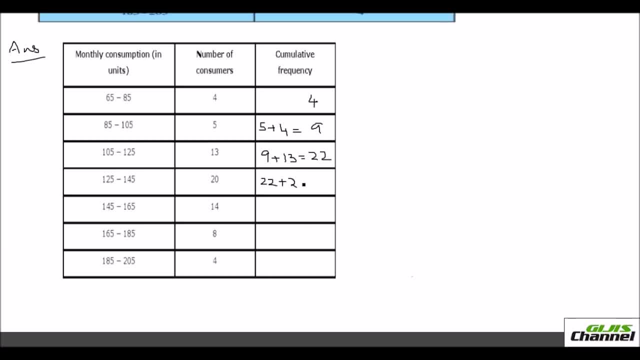 22, 22 plus 20. next number is 20, so that gives you 42. next is 42 add 14, so that's a 56. next 56 add 8, 64, 64 add 4, 68. so we have found out the cumulative frequency. if you want, you can check. 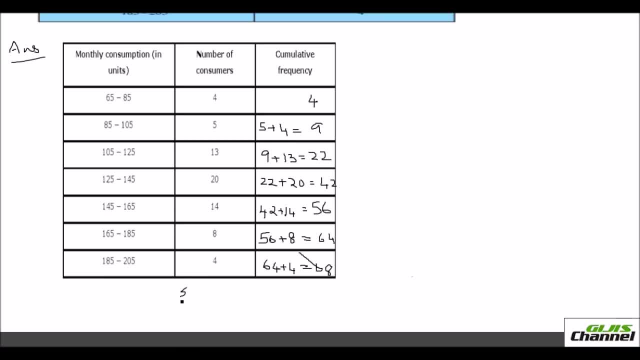 that your cumulative frequency total is right by adding up the frequency. the frequency here is 68. okay, so they match. so it is right. now you got your n. i have to do n over 2, right? see, this is different method, where you add the formula. the formula for this is the median would be. 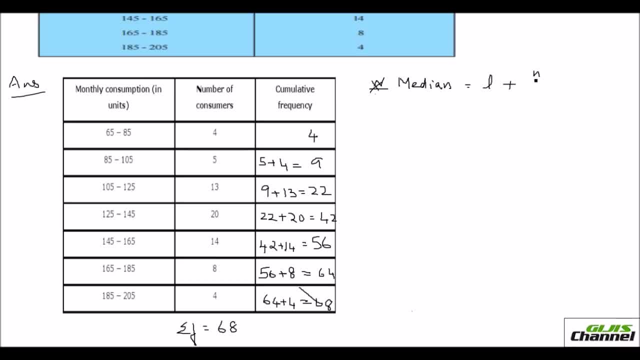 l plus n over 2. this is capital n capital n, capital n over 2 minus the cumulative frequency whole divided by the frequency close it times h. okay, first i'm going to find out n over 2. you know your n is 68, so 68 over 2. i got it as 34. i got 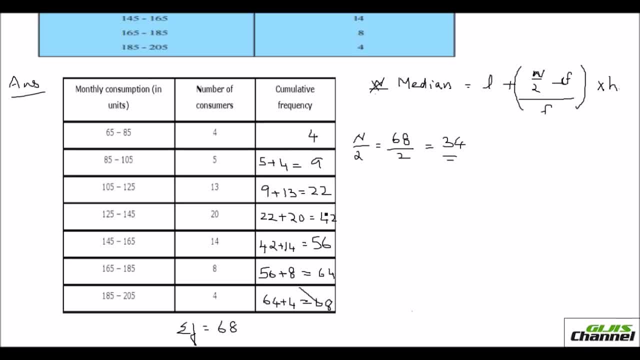 the n value now in the cumulative frequency. you don't have 34. so what you do is you just find the next number, next nearest number in the cumulative frequency. so that is 42 here. okay, this is the value you've got. so just circle this whole thing. okay, just circle this whole thing. 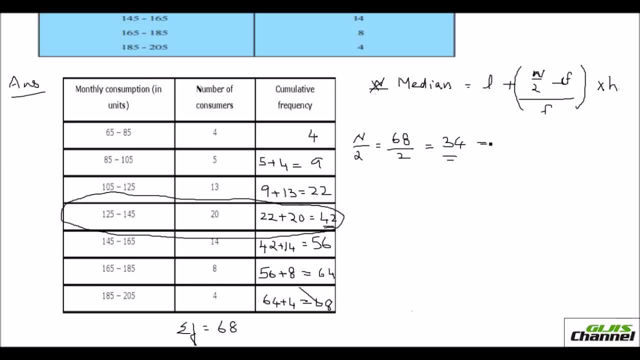 because we are going to use all these details. the number is 42, okay, and the class interval is 125 to 145, okay, your f is going to be 145, okay, so this is the value you've got. so just circle this. f and l is the lower limit, which is 125, your n by 2- you already got it as 34 and the cumulative 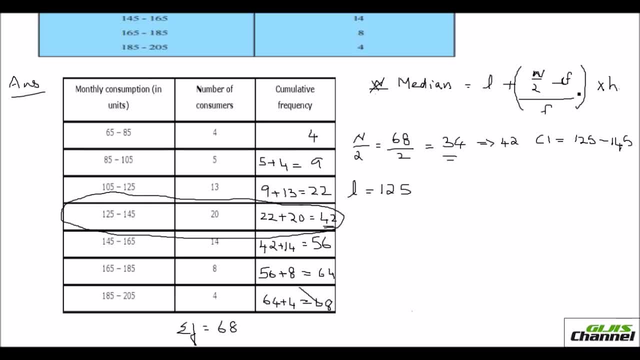 frequency is the previous cumulative frequency. okay, the cumulative frequency. so instead of writing cumulative frequency, you can even write previous cumulative frequency. so here it is this: okay, 22 is 22,. the frequency, the cumulative frequency above this marked column. okay, frequency is 22 and the frequency, just frequency, is 20,. right, this value 20, what else? and your? 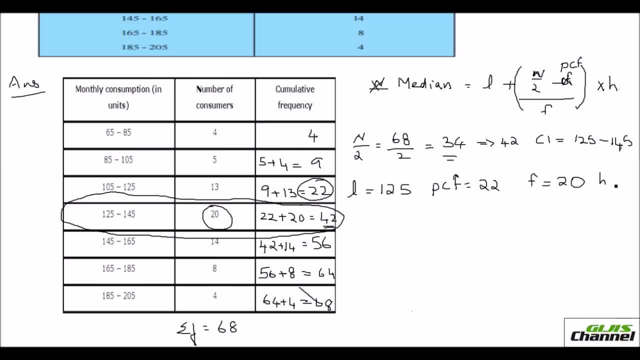 h. your h is the class size, which is also 20, now let us apply this in the formula and get the answer. so your median is equal to the lower limit, which is 125, okay, plus open the bracket n by 2 is 34 minus previous cumulative frequency is 22 divided by the cumulative.